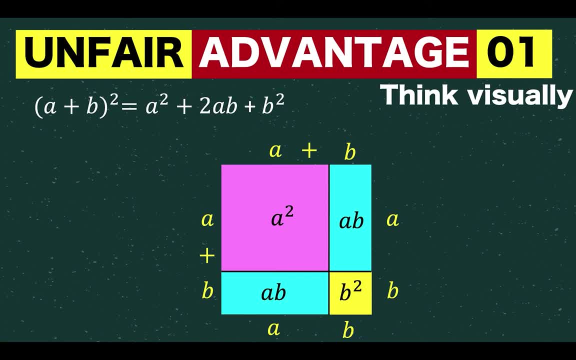 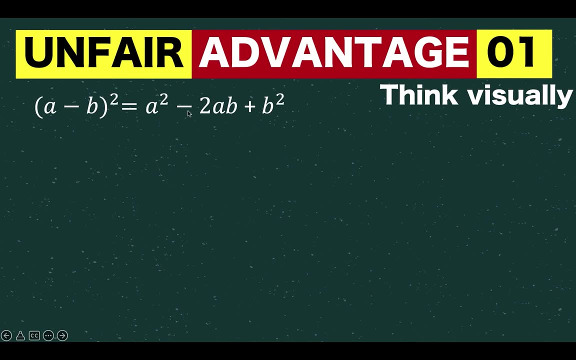 universal truth about space, and since much of engineering deals with computations in space, then this formula we know would be very crucial in the fields of engineering. Now let's say we are given this formula, the plus sign is now changed with minus sign and your teacher says: you are. 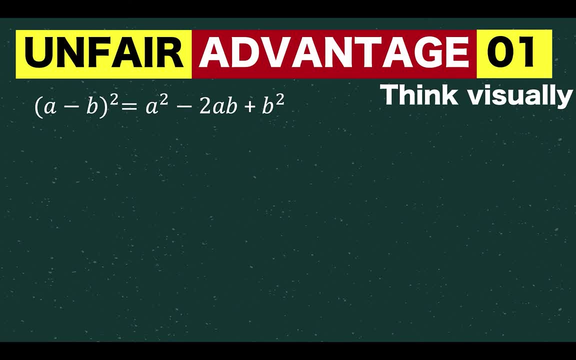 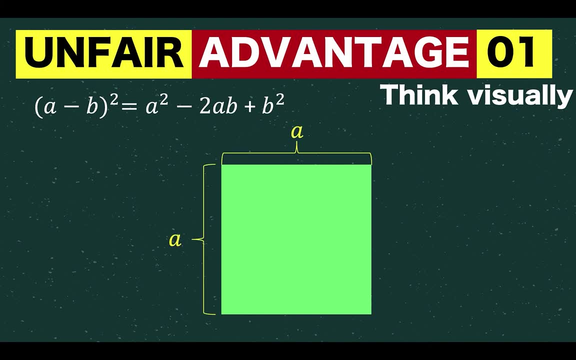 going to change this also to minus sign. Well, you can remember that, but why is that so? So let's look at the visualization again. We start with a square with a side length of a units. So a times a is a squared. that is the area of this green. 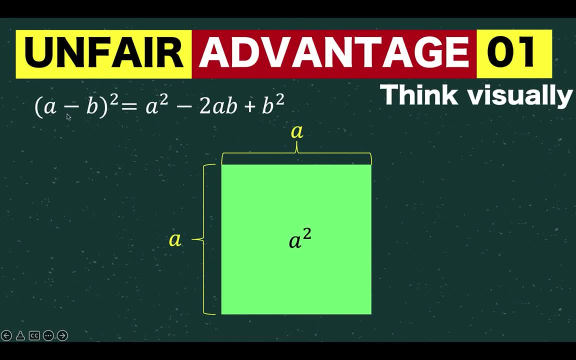 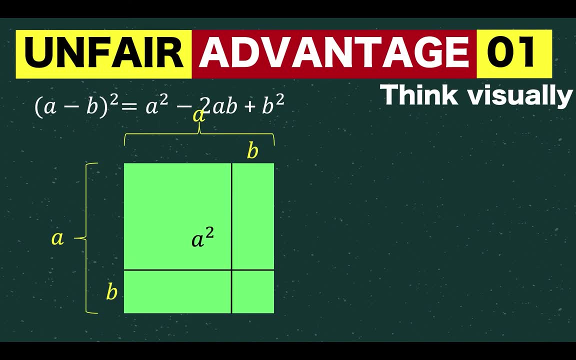 square. Now, since here the side length of the square is a minus b, that means we are going to subtract some quantity of magnitude b from this side length of a, and let's do that. So this is now our result: The a minus b squared would now be this blue square. The length of this blue square is a deducted by. 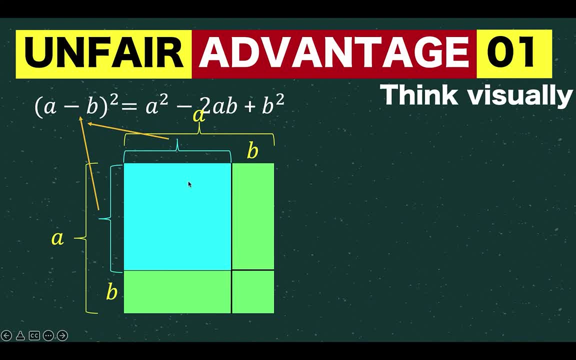 this b. So this is square of a minus b. therefore it talks about the area of this blue square. And looking at now the composition of our squares and rectangles here, here is what we found: The square of a minus b. that means the area of this blue. 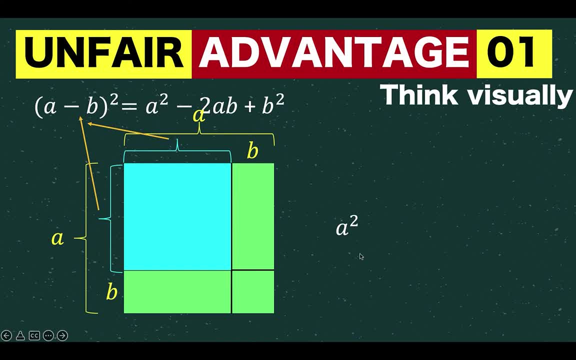 square cannot be computed this way. You start with a green square with an area of a squared, but we are going to deduct the area of this rectangle which is minus a b and the area also of this other rectangle at the bottom which is again negative a b. But wait a minute, notice that we counted the. 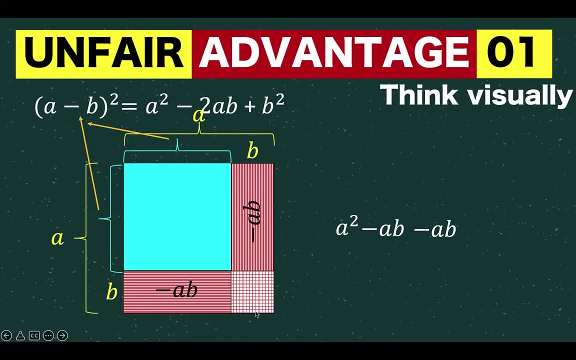 this area twice, because that's already computed in the first rectangle and that's computed again in the second rectangle. So we need to return back this part that was counted twice and so we need to add that part that was subtracted twice and we now have this plus b squared And simplifying this. 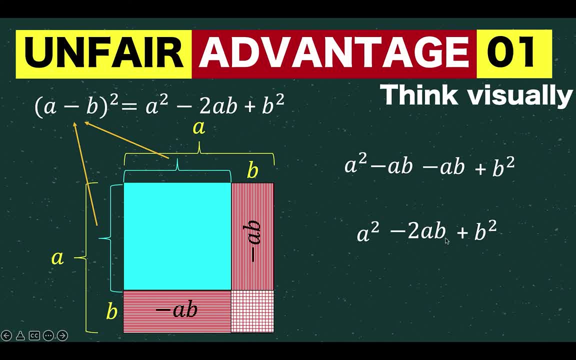 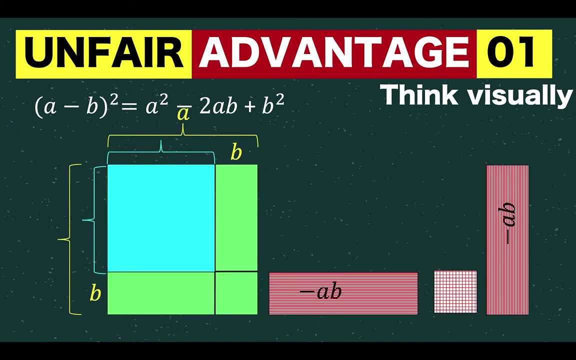 we arrive at a squared minus 2, a b plus b squared, which is now this right side of the equation. Now, after we are looking at this is you can see how these components are interrelated. You can see that this part was indeed counted twice. So if we remove that, we now have 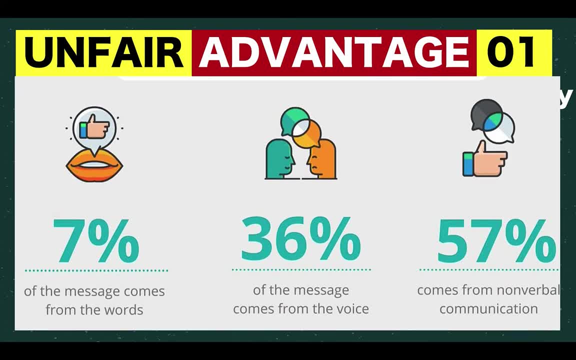 this figure. Now here's another idea. According to research, seven percent of communication is in the form of words and the rest in the form of voice and non-verbal communication. So if you are the student that rely heavily on memorizing in words these formulas, you are missing a lot of. 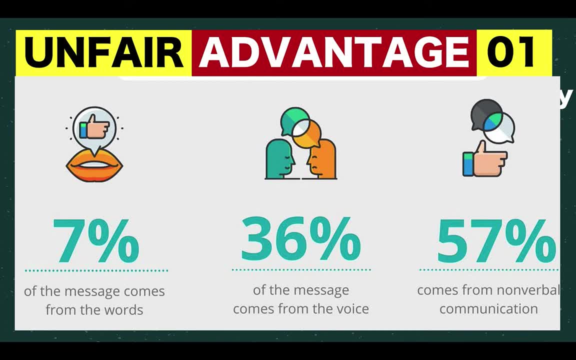 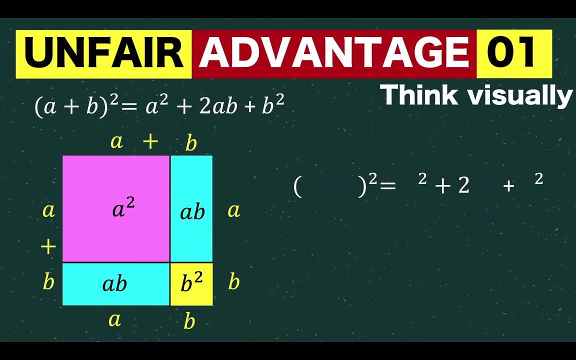 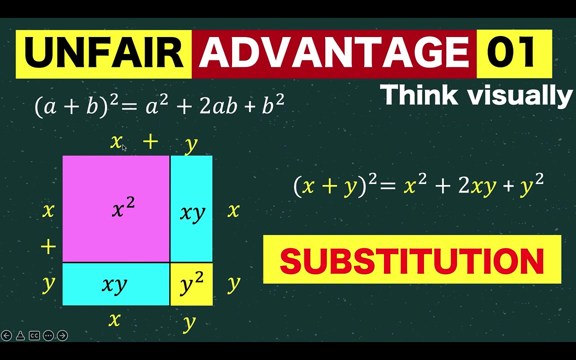 opportunities to be at par with the more superior students using mathematics. Now, the good thing about mathematics is that once you establish that something is true, then you can just use the concept of substitution to apply the formula in specific instances. For example, in this formula, it doesn't matter whether I use a or b or I use letters x or y If I replace a by x and b by y. 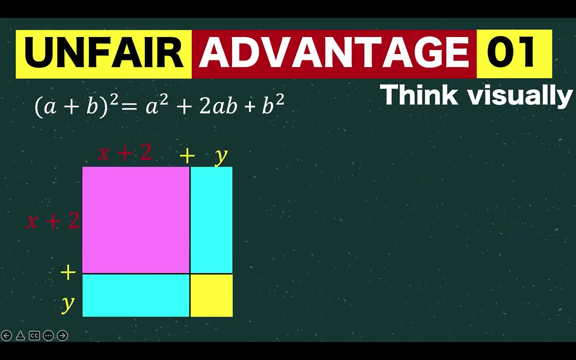 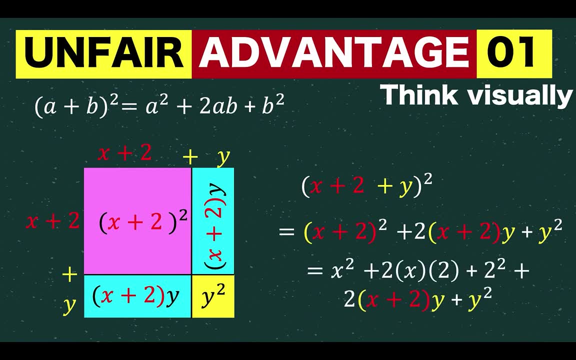 then this formula is still true. In fact, I can even replace this a by a binomial x plus 2, and still applies, And that becomes like this: Notice that this part is just substitution. I did not perform any computations, I just apply the formula by substituting this x plus 2 to a, And only in. 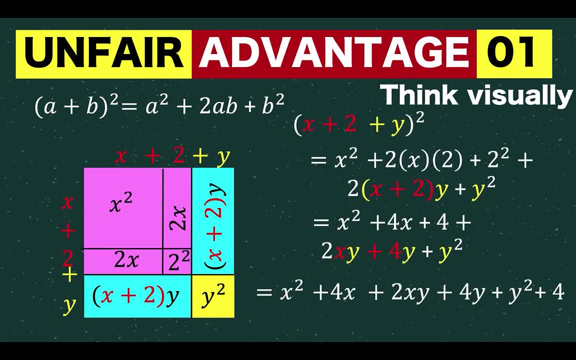 this last two steps when I perform some minor computation to come up with the final answer. So, contrary to most belief, math is not just about computation. Math is a way of thinking, Math is the language of the universe And if you think of mathematics just as 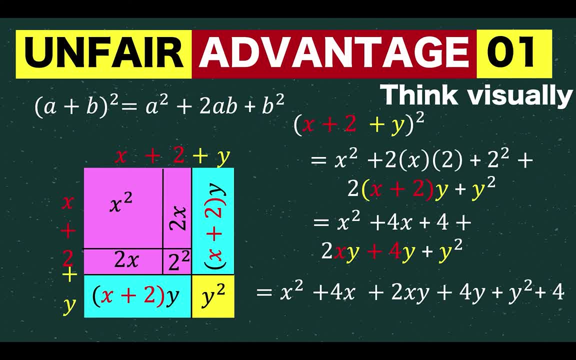 a computation. you are thinking of math as just arithmetic, And computers can perform this task much better than human beings. So in mathematics we are not so much about computation. We are after learning this universal truth about the universe that's stated in mathematical language.